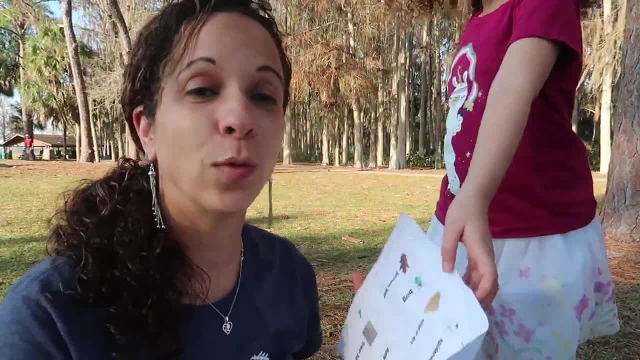 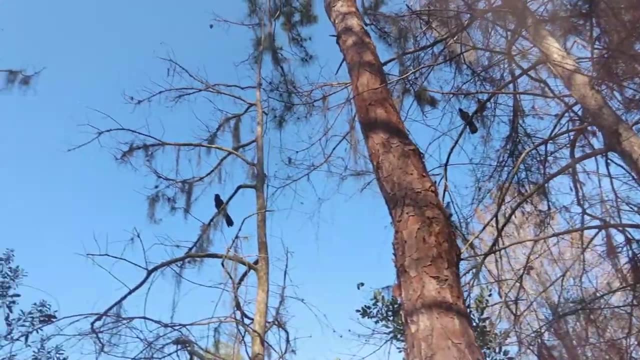 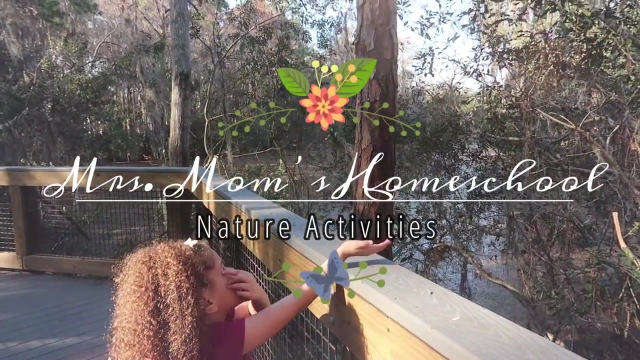 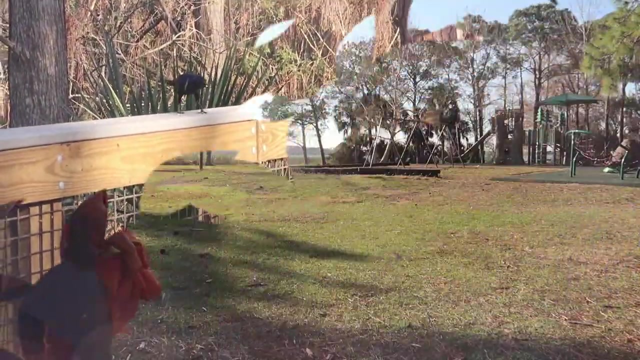 Are you looking to incorporate some nature study into your homeschool? Well, today I'm going to share with you some cool ideas that we have that you can do outdoors with your kids. I previously made a video on being in a homeschool rut. Some of the activities. 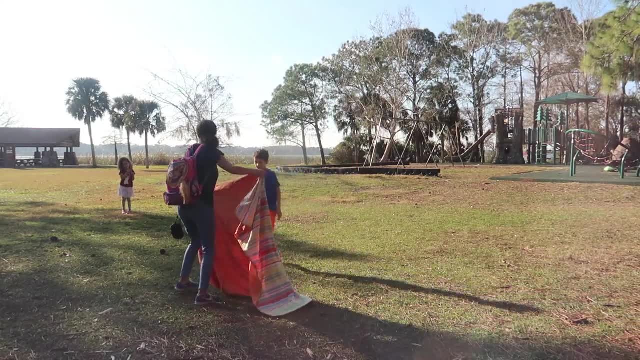 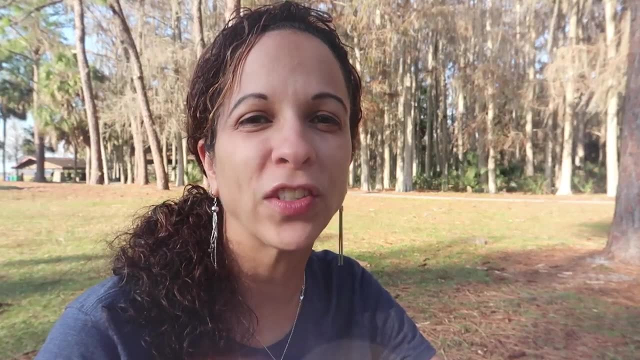 that I mentioned were to help you guys get out of the classroom and bring some joy into your homeschool, And one of those things was getting out into nature and doing some educational activities outside. So we're here at the park today doing some of those activities. Right now I have a little one playing at the 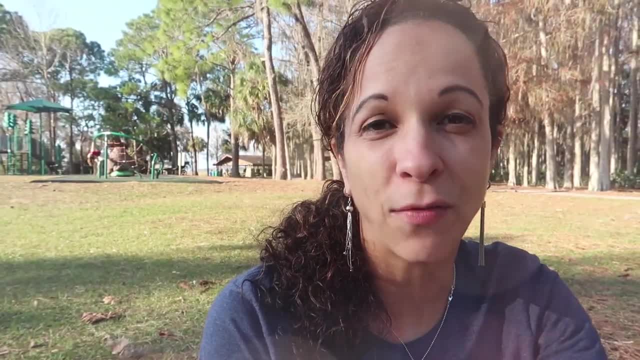 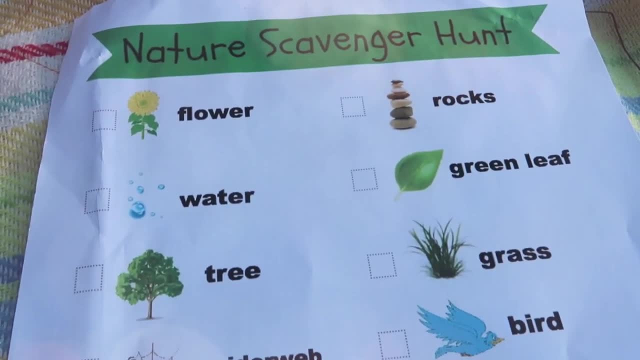 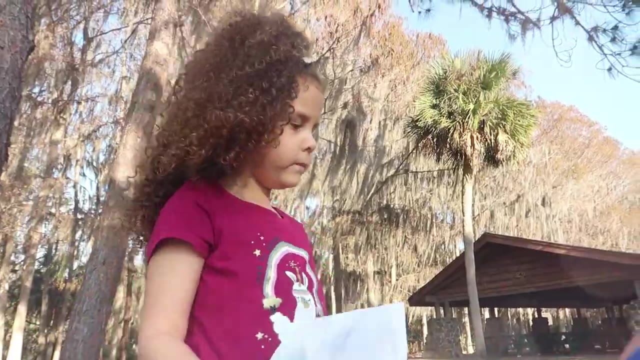 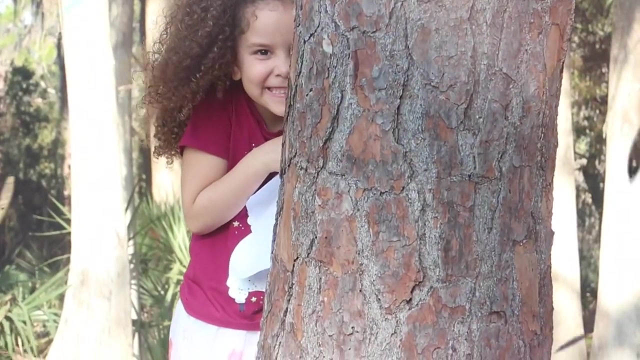 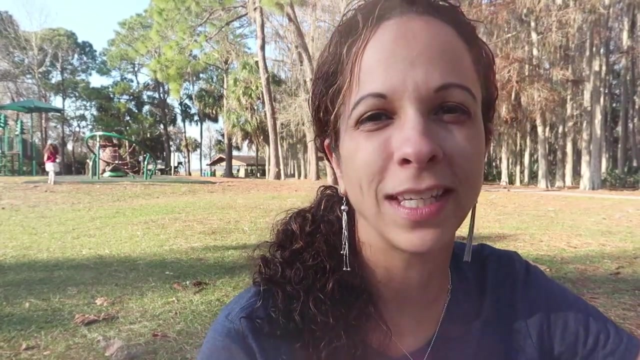 playground and I have another one doing a scavenger hunt. So I printed the scavenger hunt off of the internet and I have my kids going around with my camera to take pictures of all the things that they can find. I have to come up with a little prize to give them when we get home. I have a 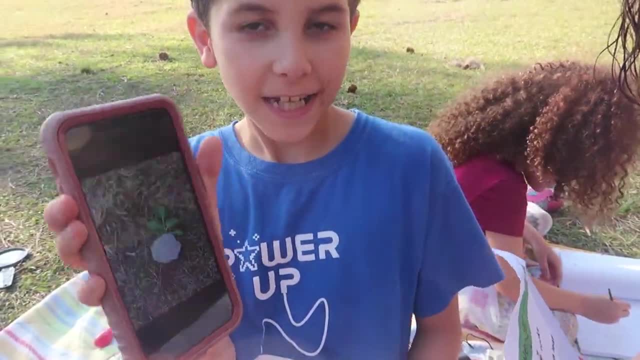 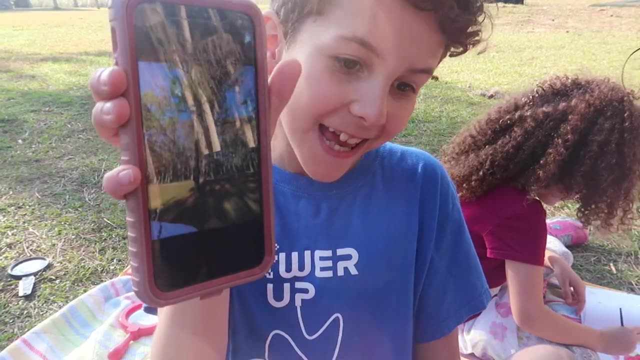 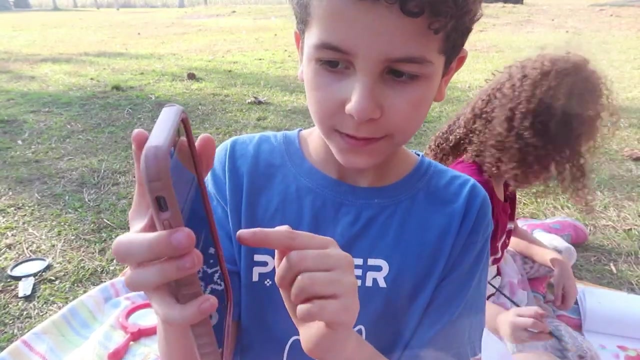 flower, Yes, flower, I have them all in order. Water Water- Nice Tree Trees, Not so trees. Spider web: We didn't get. did you get that one Spider web? Nice, good job. Another activity you could do is bring some watercolors and a nature. 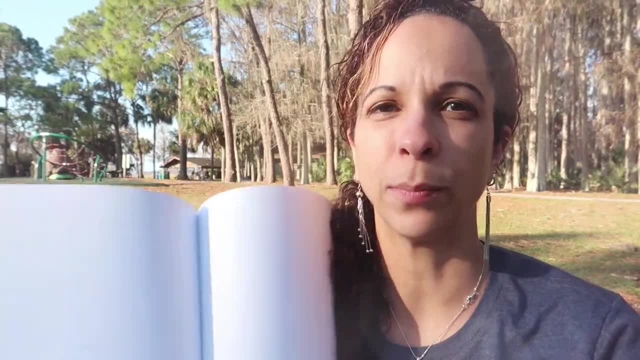 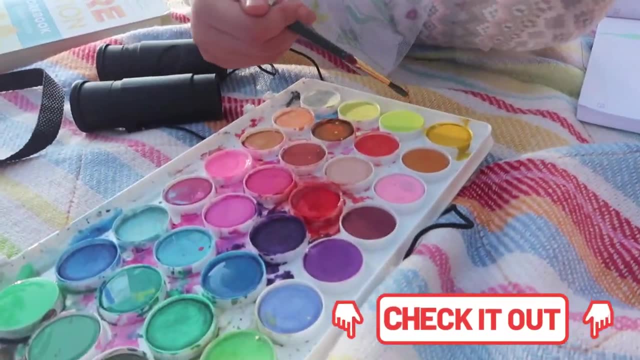 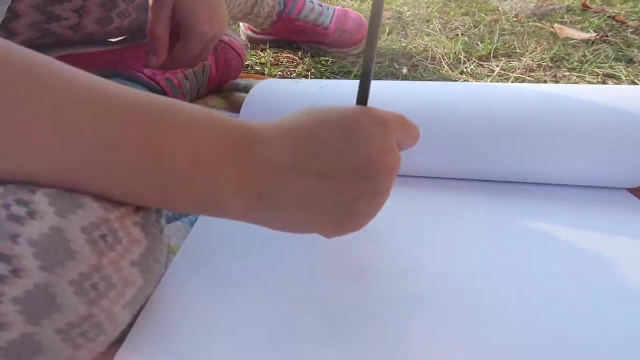 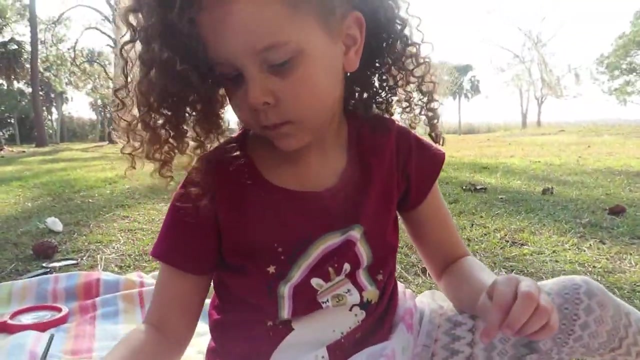 journal. We got these off of Amazon and they're just blank pages inside and your kids can paint a picture or draw a picture that they see in nature in their journals. One way to rinse off your paintbrushes is to have a Ziploc bag and fill it with a little. 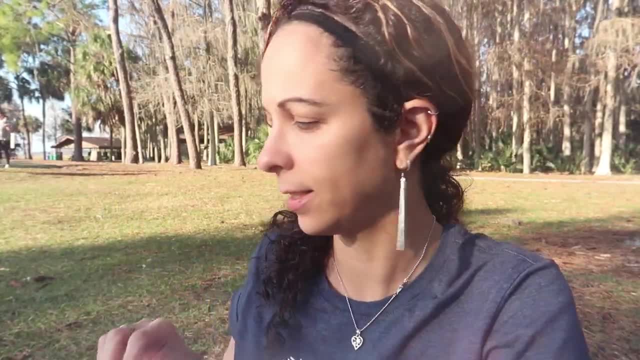 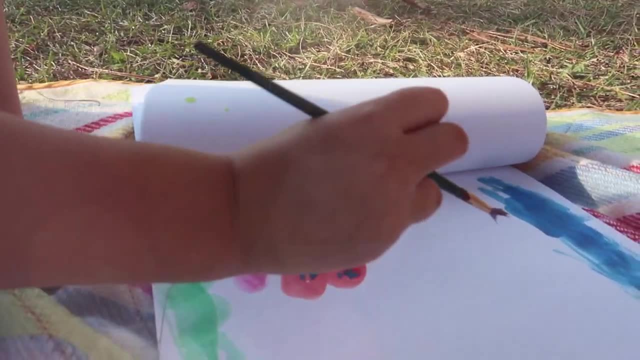 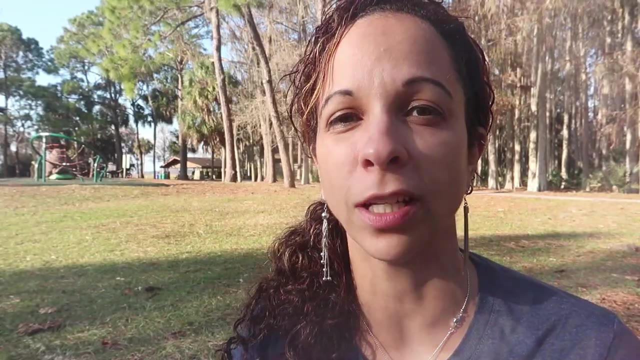 bit of water and they can swivel around the paintbrush in the Ziploc bag. There you go. Another thing you guys can do with a nature hunt is to gather some of the materials and make a nature collage. You can also have your kids grab a bunch of materials and make some nature critters. 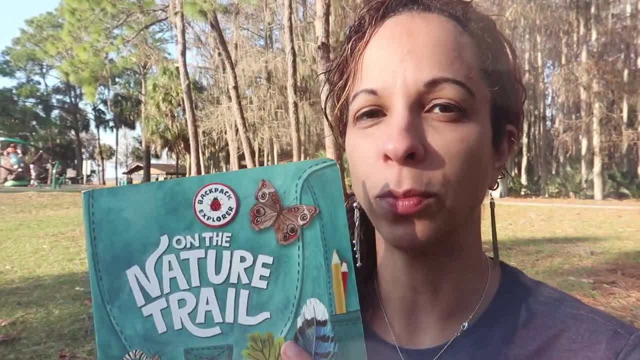 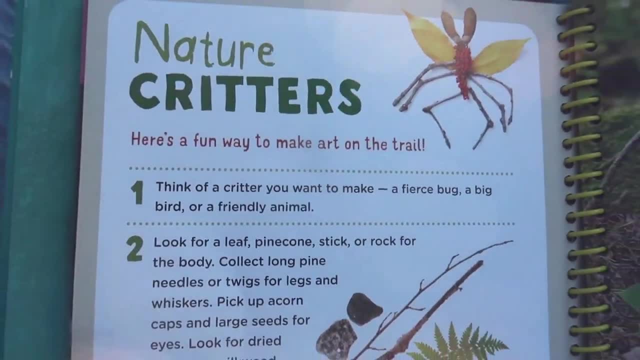 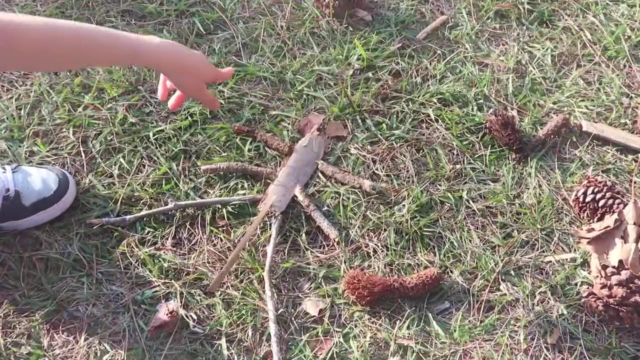 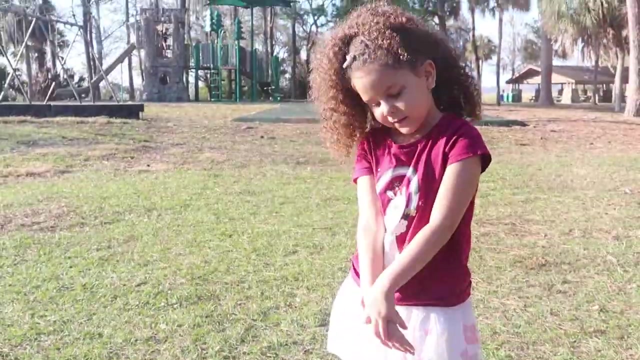 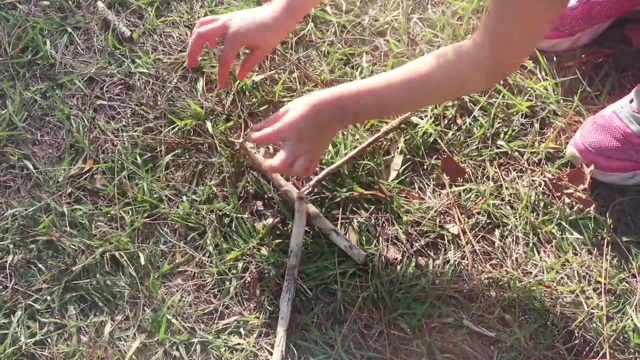 like these that we found in this On the Nature Trail book. I like it Looks creepy. Let me see yours. Tell me again: This one is a fly. Let's look at it. These are the wings, These are the antennas, These are the eyes. 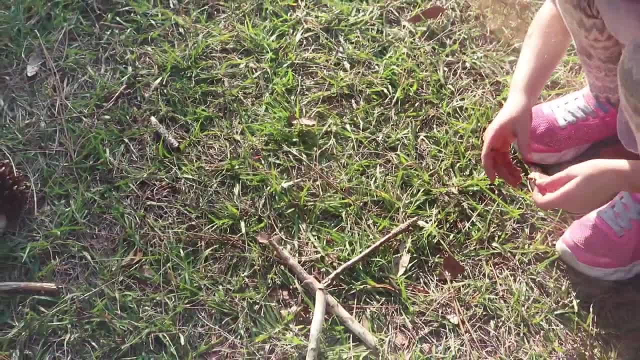 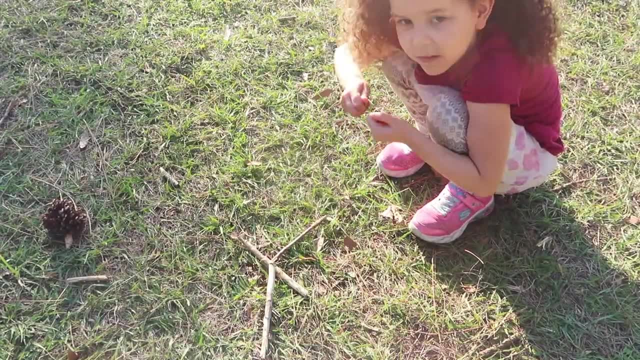 Great job guys. And then I can add like this: Like a little extra little leg, Okay. And then I can add: like this: Like a little extra little leg, Okay. And then I can add like this: Like a little extra little leg. 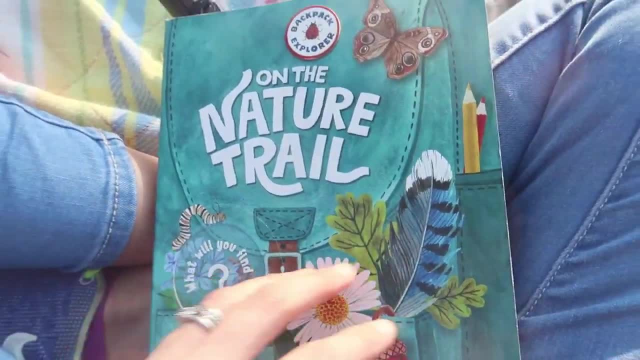 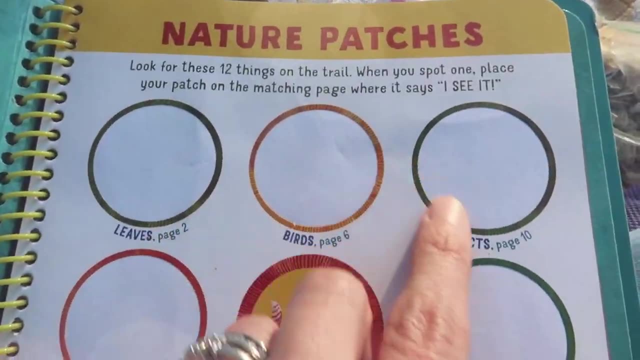 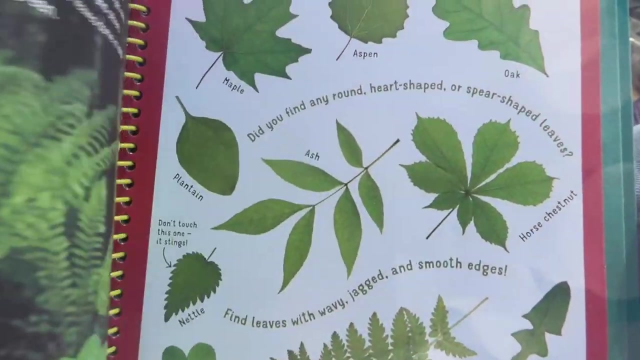 My perfect bug Love it. This On the Trail journal is awesome. It's by Backpack Explorer and they have a couple of different ones. They have different patches that you can use and when you complete a section you can put your patches there. For example, this section is about leaves. 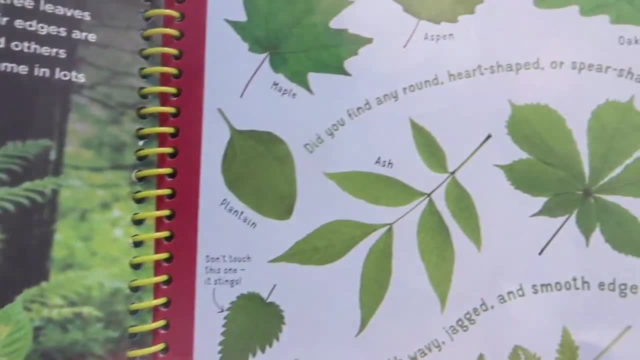 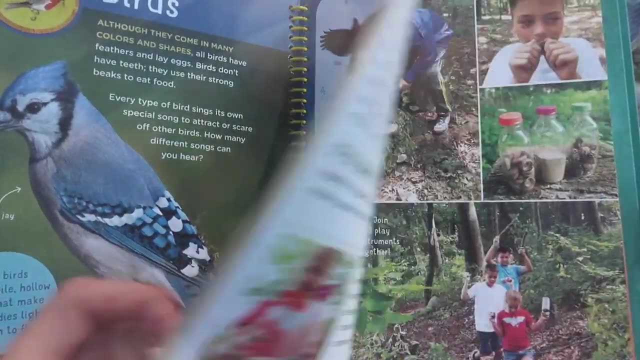 We studied the leaves and then we added our patch. there You have things from leaves, You have things from plants. You have things from plants. You have things from trees and birds and insects and slugs and lots of different activities. You have things from leaves and then you have things like this in the top corner of this: 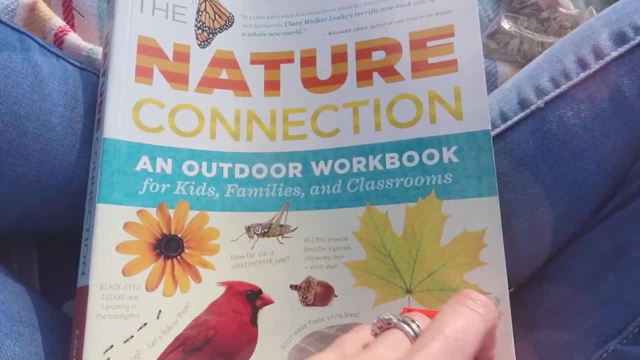 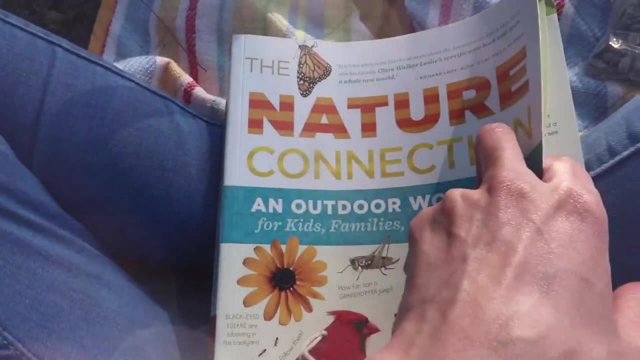 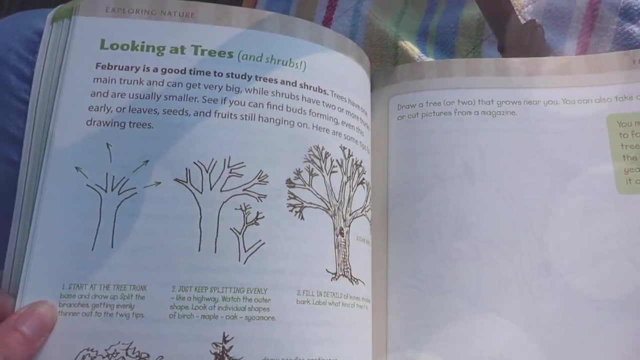 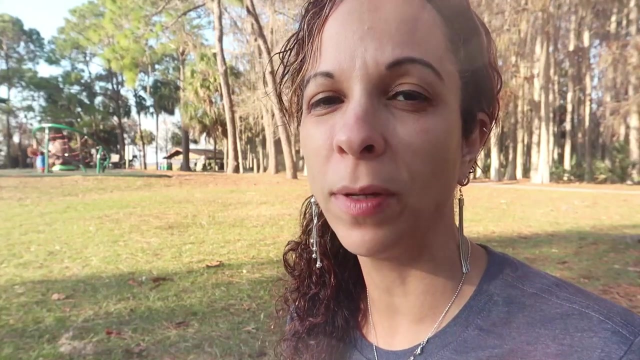 section. For the next section, you have things like this: One of my favorite books is The Nature Connection. This is an outdoor workbook and this has a bunch of different activities that you canат and it's also a journal for the kids. Keep your bag clean.